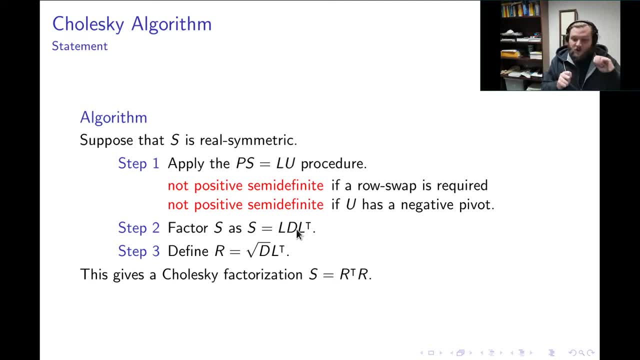 because in this situation the diagonal of U will not have any negative numbers on it. So I can define R as the square root of D times L transpose, and this is guaranteed to give me a Cholesky factorization. S equals R transpose times R. The reason that this R works is because 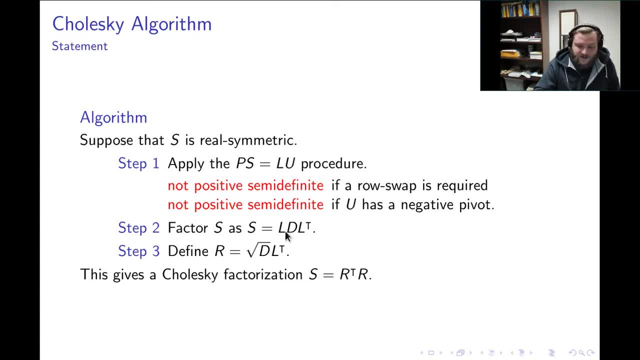 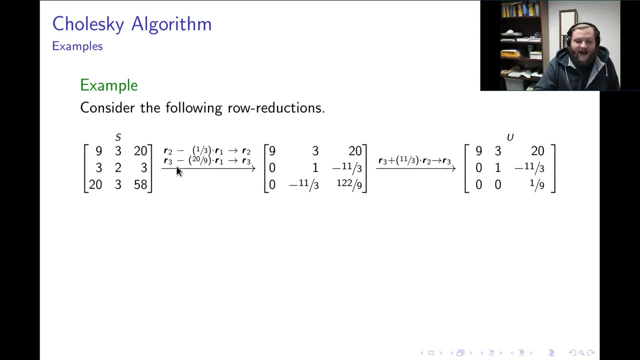 defining R as root D times L transpose allows me to split up S as the gramian of R, because S is L times D times L transpose. So let's see this in action. Here I have a three by three real symmetric matrix S and I've applied the PS equals LU. 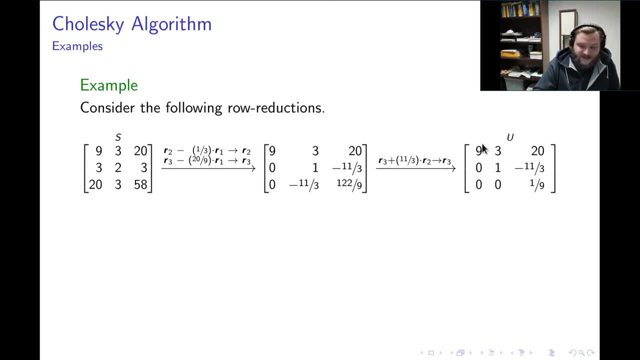 procedure to row reduce S to U here. Now, along the way I didn't need a row swap and also I end up with no negative numbers on the diagonal of U here. So this matrix, S, is positive semi-definite. In fact, when I get to U I see that there are no zero pivots, so S is actually positive definite. 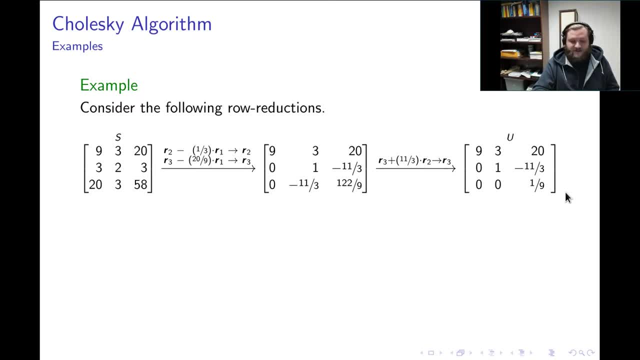 So how do I produce a Koleski factorization given this setup? Well, remember our formula for R and S equals R transpose times R is R equals the square root of D times L transpose D. here is the diagonal matrix, whose diagonal entries consist of the pivots in U, So D would have diagonal entries. 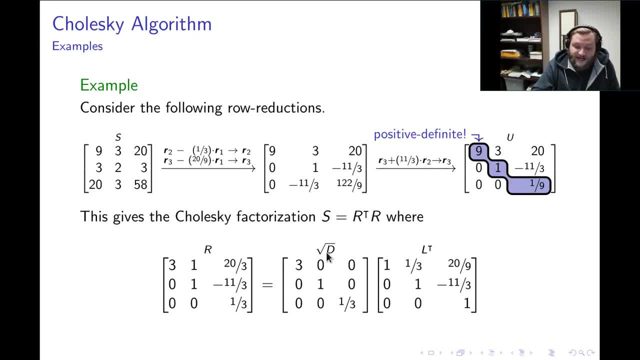 9,, 1, and 1- 9th. So when I take the square root of D, I get the square root of 9, which is 3,, the square root of 1, which is 1, and the square root of 1- 9th, which is 1- 3rd. Then I have L transpose where L. 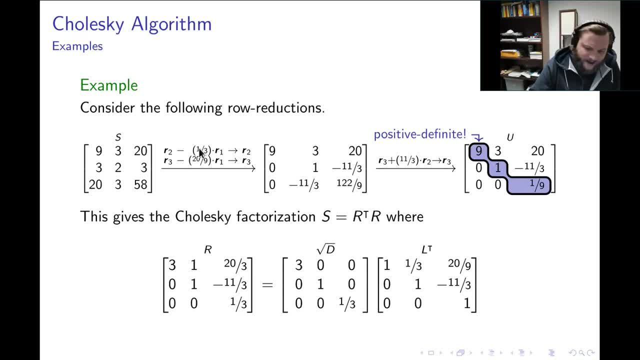 came from LU where I inserted the negatives of my multipliers into a lower triangular matrix, And so this gives me my Koleski factorization. S is positive definite here, so I could factor it as LDL transpose where D has a positive diagonal. and then I can go further and say S is also the Gramian of an. 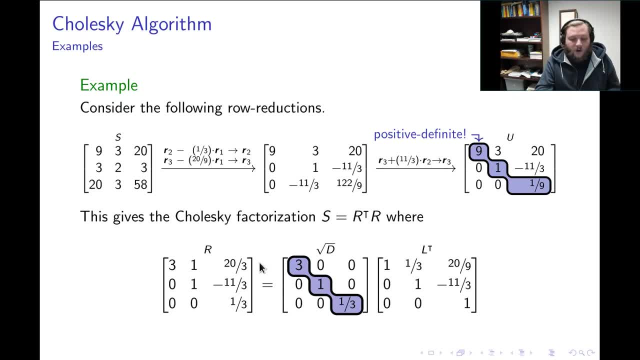 upper triangular R with positive diagonal, where R here is root, D times L transpose. So here I see, R is indeed upper triangular with positive diagonal. So that's Koleski factorizations.